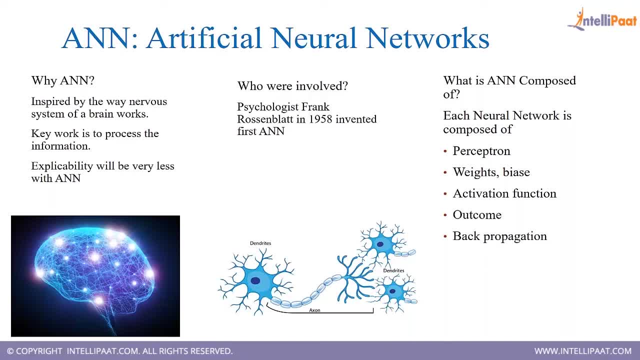 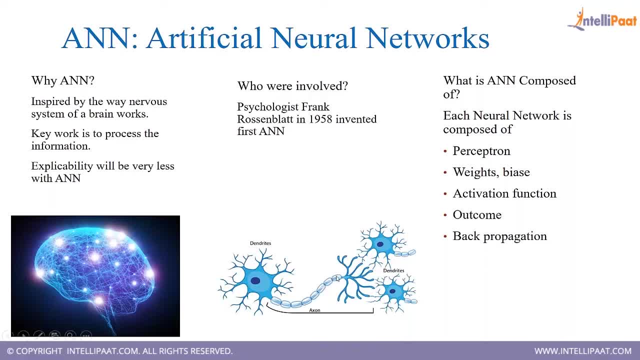 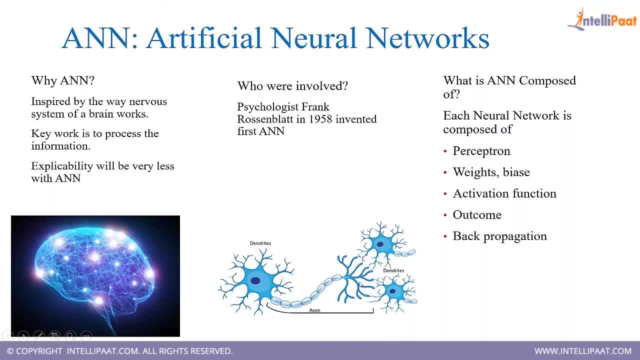 it passes on to the next layer. You can see next neurons nearby, so that all things goes like this. So as people mimic and say human like inhuman work, let's say someone is just. Women's brain works very faster as compared to men's brain, right, 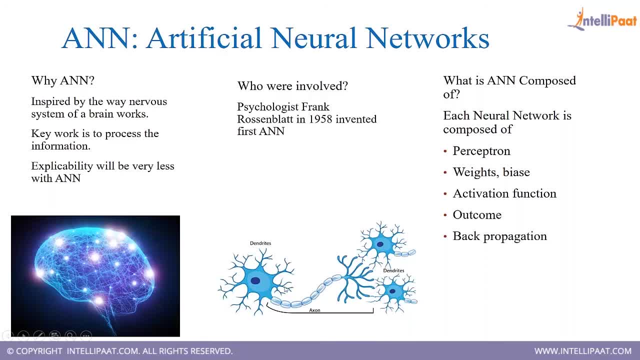 The way the signals proceed from here and there. it is very fast in women's as compared to men's. The thing is, it totally depends on the way the computation takes place or the decisions taking place at this point, and the signals will be passed to the next layer. 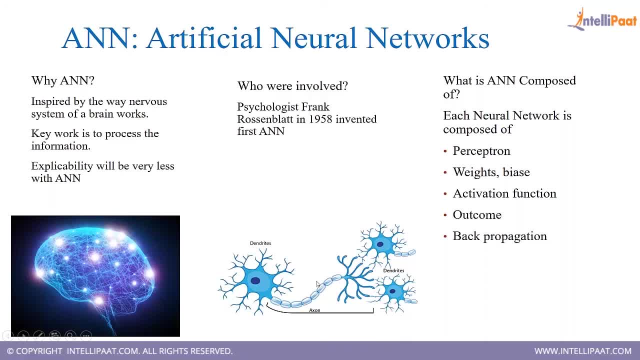 Similarly, you have architecture for artificial neural network right. What actually artificial neural network was, it was like, let's say, three different whys for whom why and who were involved and what is actually the component of TN, right? So Franklin Rosenberg in 1958,: 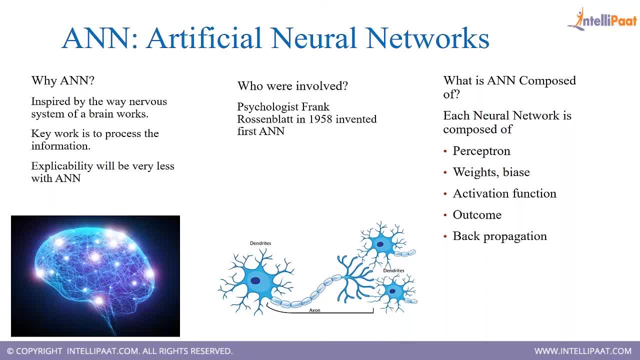 was the one who was the author for artificial neural networks and he did all this research and tried to mimic the human brain right And build a model or a machine learning model. The components for the ANN is the perceptron, the human neuron weights associated with that. 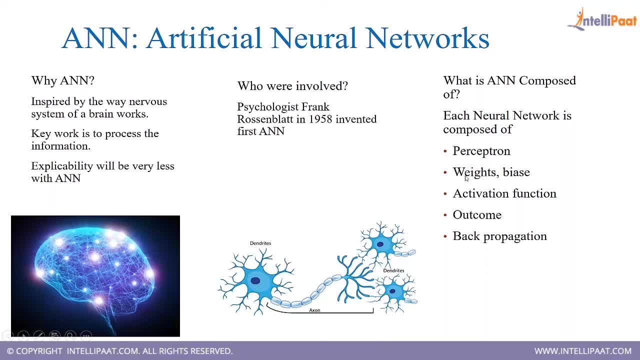 the importance actually weight provides signifies the importance of each neuron, Each parameter, right? Let's say you have a lot of parameters in it. What is the weight associated with that? What weight agent consists? So that is very important. 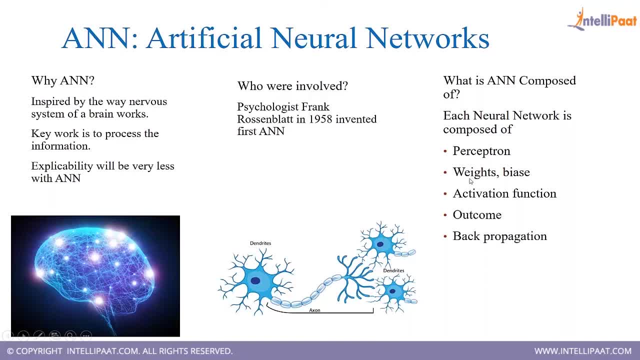 Ultimately, in the neural networks, what you learn is: which is weight associated with each input, parameter Biases to control the error factor there, the unknown error factor, Activation function. So, at each neuron, what makes this to be activated? What makes it to be inactive? 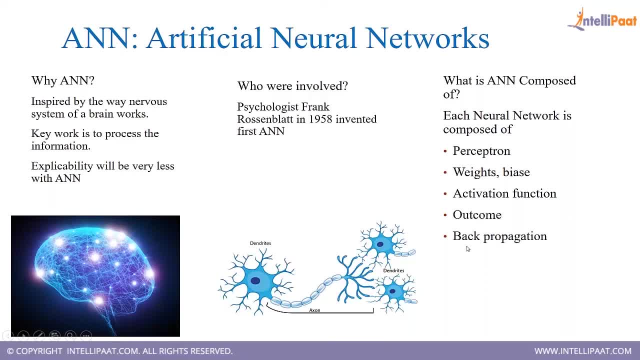 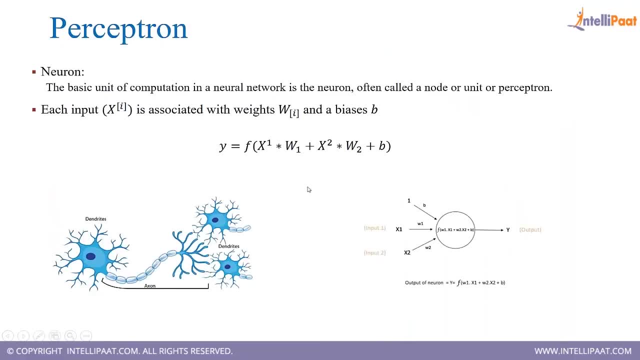 Like that, right, Those things. The outcome and back propagation is another concept there. So we will be looking today in this area, right, Let's say what actually a single perceptron or a neuron does. Neuron is a biological term for a given single basic unit of your brain, right? 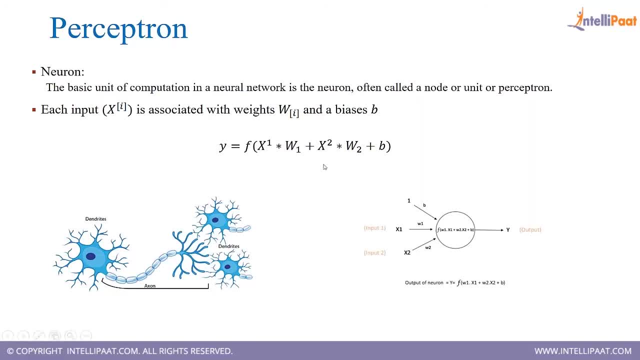 Perceptron is a mathematical representation of your neuron, right? That's where I called it as perceptron, or you can call it as a neuron also. That's my terminology difference in there. So you have a mathematical representation of all this. 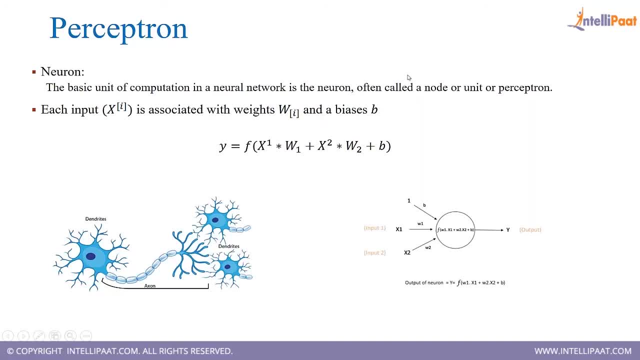 You say perceptron or neuron, or people call it as node or unit. It depends right. All three or four points to the same thing. So neuron is the basic unit of the computation in neural net. Right It often called as node, unit or perceptron. 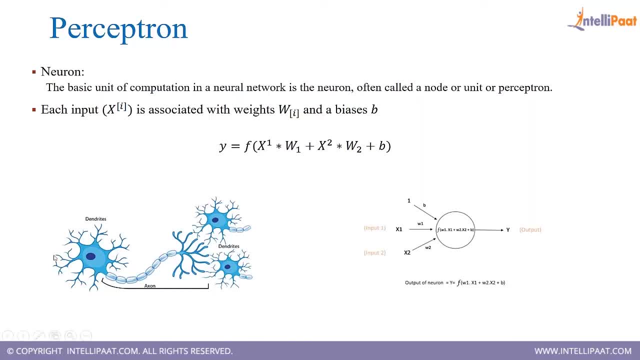 So there are a lot of input for that. Let's say, these are the input areas. I will just pull over those. Yeah, So if you see here from here, So if you see this from this, I get X1.. 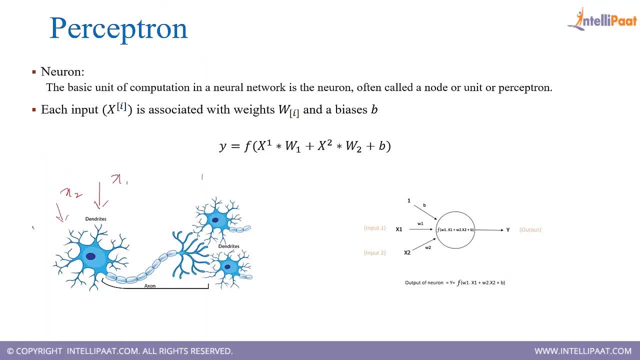 From this, I may get X2.. From this, I may get X3.. Right, This is how I feed my input values. Alright, So this is how, if you consider this one as your neuron, is what your this area? What you are doing is you are providing them. the input values are X1, X2, and so on. 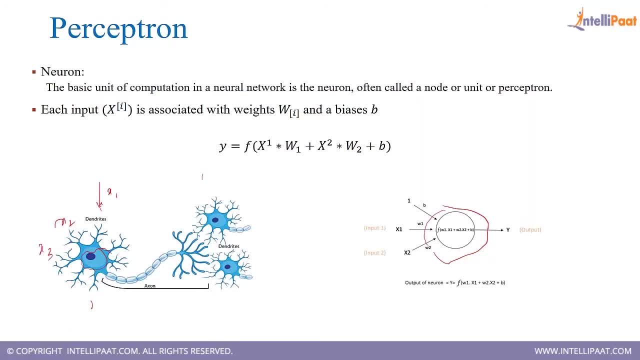 X3., X4., X5. Xn. These are the input parameters for you which are associated with some weights. Weightage in the sense: this has some weightage. This has some weightage of factor weight. 2. This has some weightage, factor with 3.. 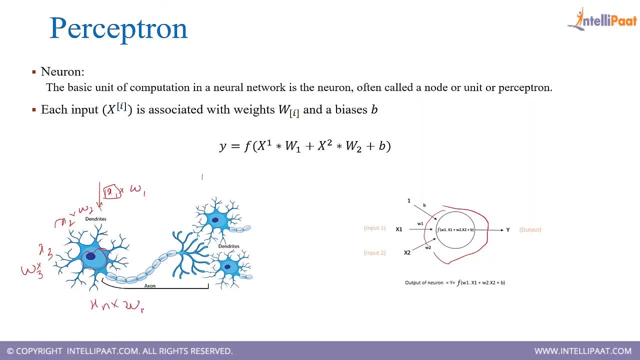 And this has a weightage factor of W of n, Right. Each contributes to a function And gets their associated input as well as their weights. How significantly this input value is Right. Those things are there And, with some constant, Constant value, are to maintain the error factor and all those things. 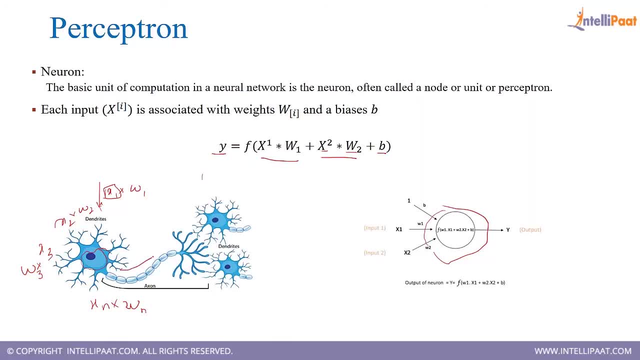 This gives you your Y value. What should go for the next? actually? Okay, That is what is being represented here, The real format of a neuron, Right? So if you see, it is a function of these stuff, which consists of weight and input as well. 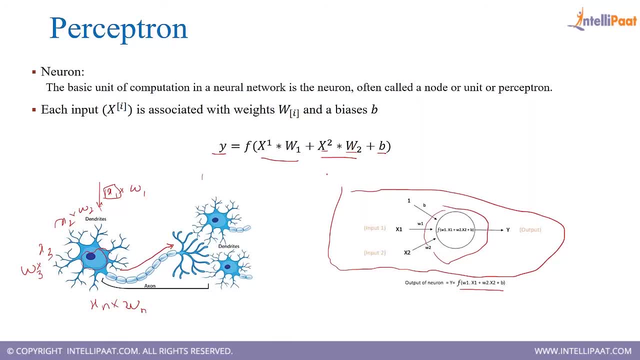 as weight And then biases. Okay, This is one important stuff we need to remember. as of neuron, What actually it consists of. Each neuron will give you a Y value, taking various input factor and the weight and biases. Some point, you get biases from here. 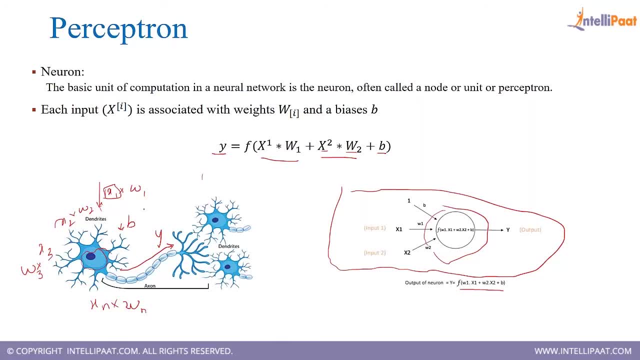 Whatever It is. If you want to just analyze, It will be like this And the other stuff are like. in the neuron It happens like this: If you see the data in the real time, It can be of two different varieties of the data. 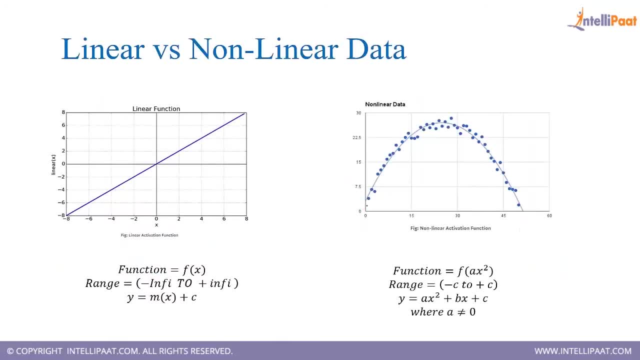 Data can be a linear format, For example Linear in the sense. Probably you might have learnt in linear algebra Mx plus C, Right, This was the slope function for linear, Linear, Linear, Linear, Linear, Linear, Linear. 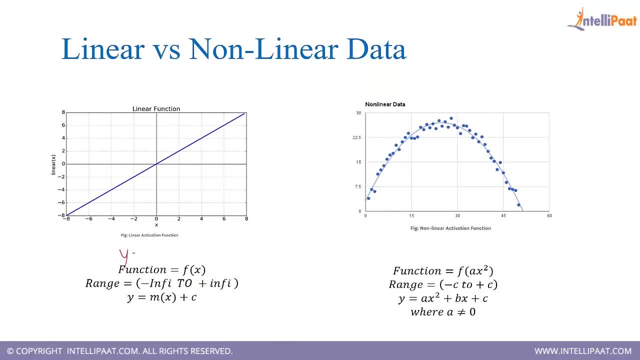 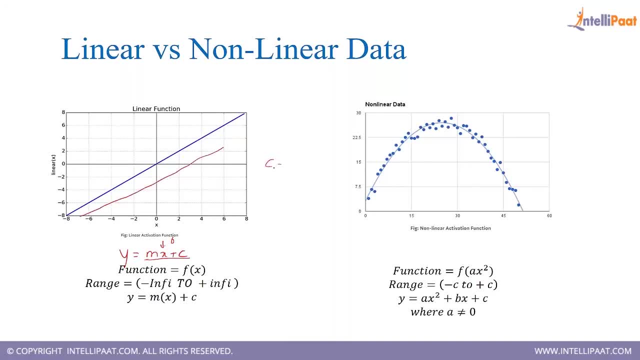 Then graph would go like this: If C value is somewhere around minus five, something Right, Minus five or so, So at that point of time Your constant would be here, And then M value is your slope factor And X is your coordinate. 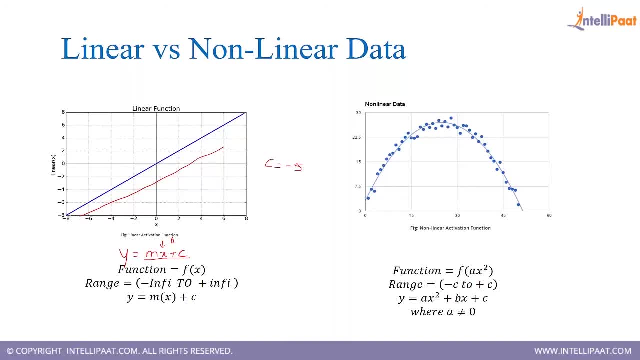 X time how you should write X goes and all this. actually, yeah, the graph would start something like this: so here your x factor, c factor is in in this blue line. your c factor is minus 8, like that. okay, so just for a reference, i've just given that. yeah, so so linear for an example, what i'll give a real-time example for. 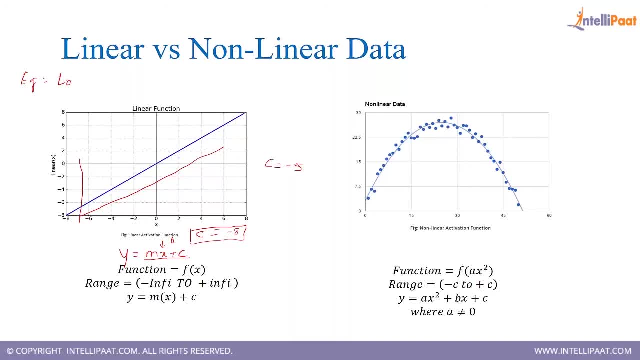 this right. what happens is you are trying to get a loan right. this is your data set, loan prediction stuff. okay, what we are trying to say is: this is your y value, which says decision to be taken care based on the loan. this is your- probably name, or so, whatever the values, 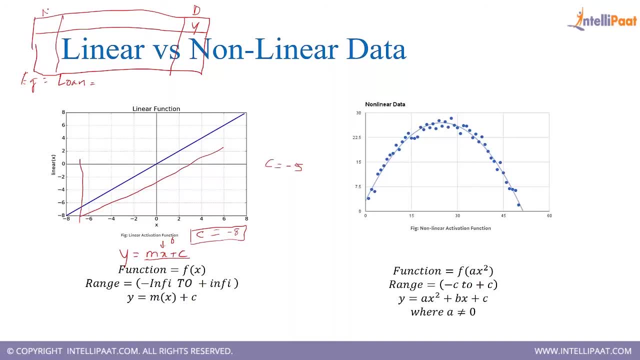 okay, name and okay name, then age, then your salary, then your spouse working status, then your credit card. based on that, you are taking decision either to give loan or to not, to give. right, this is your binary class classification problem. okay, okay, okay, your salary, age and all those things made some impact on it, so you will end up with a function. 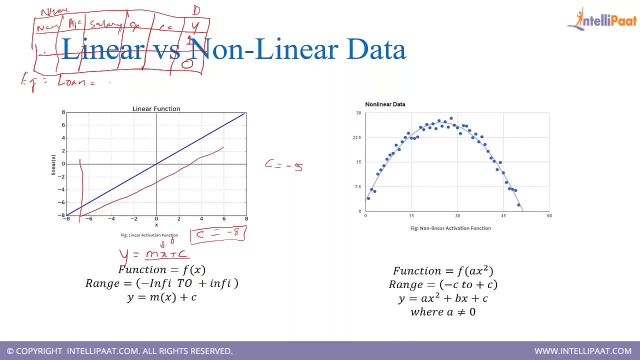 which says, if your name you can drop it or something you can drop it, age associated with that some some significance. saying that age would give among the loan to be given, as your hundred percent, which is you say, age would uh, implies you with a 20 percent. 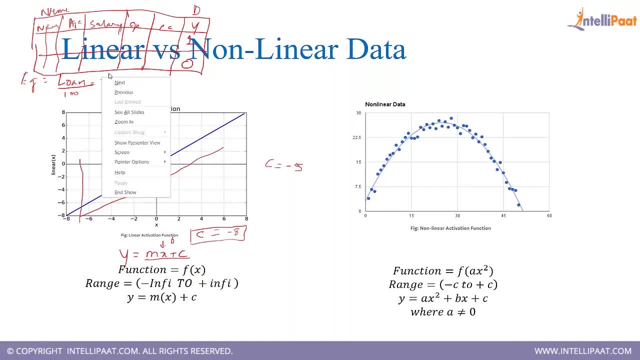 age right: 20 percent chances, uh. weightage of loan then: 0.1 i mean 30 percent chances. of 30 percent chances i mean weightage of your salary sheet: Wealth ici plus somewhere along your spouse working would be like 10% to give your uh. 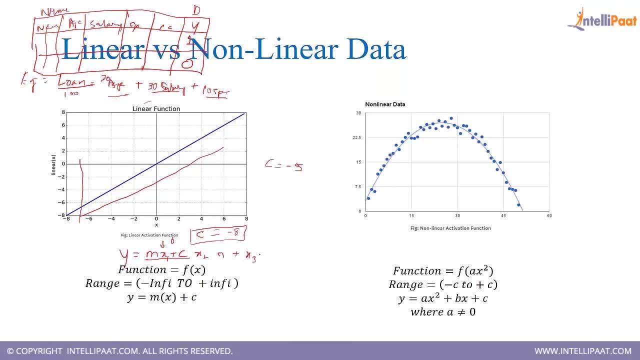 loan status. each has some weights associated with that and you don't have nonlinearity in this. you make a equation such like mx1 plus x2 into m2, like that right: m2 plus x3, m3, x3, m3 and so forth and so on. this made you a equation, simple, linear regression problem. 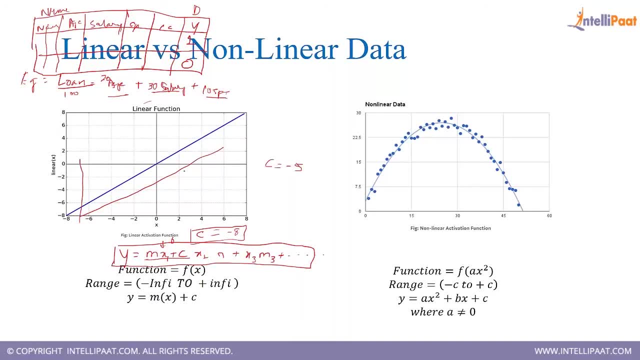 got it. it creates a simple linear regression, but when it this forms a linear, linear data, this forms a linear data, but sometimes there will not be a linearity in the data. it can be like non-linear data. you can have any other patterns in it. that particular data, those particular data. 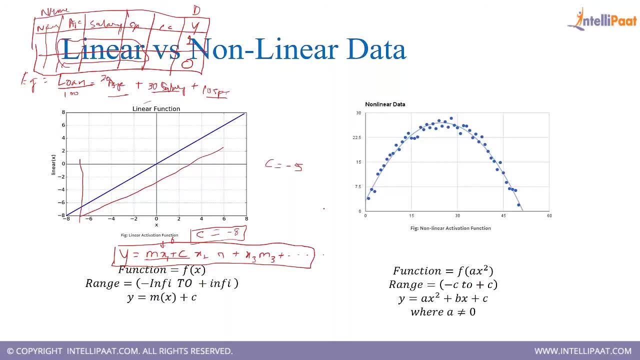 can be considered as your non-linear. so probably you cannot find the significance when you try to segregate between loan giver or non-loan giver. you cannot segregate them, this class, you cannot segregate by by this linearity differentiating. if you provide this line, those are coming about. 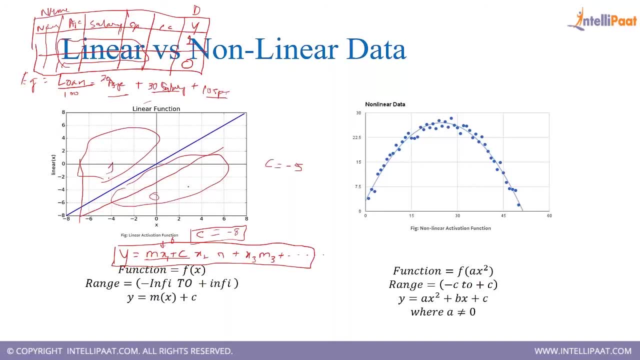 you can give loan. those are coming below this. you cannot give sort of like classificate but in this case you need your. it will be like you can give loan. those are coming below this. you cannot give sort of like classificate but you can give loan. those are coming below this. you cannot give sort of like classificate, but 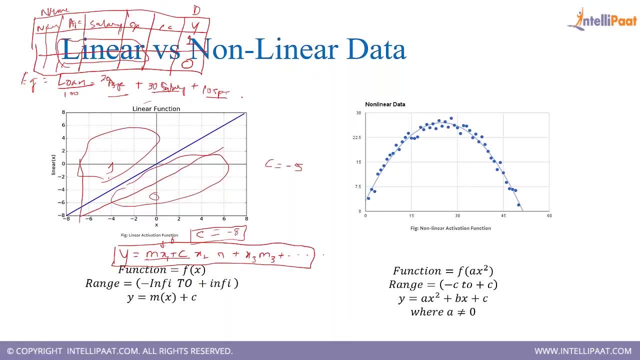 you need to learn the data in a different way. so in mn you have lot of other algorithm for handling this log exponential and all those things you use in order to make this one to a linear form. first you make the exponential factor and then, uh, log likelihood. you, you use that right log likelihood. 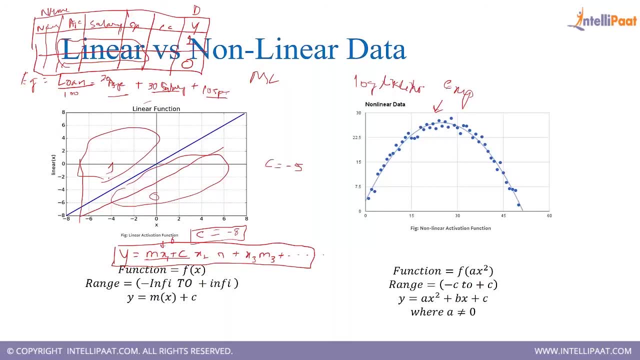 you, you, you use that right log likelihood, you use those, and then you make this, transform this into Wilson, and then you make this, transform this into a linear format, and then you apply linear regression also, so so that it will be like fitting this equation, or else you provide this non-linearity. 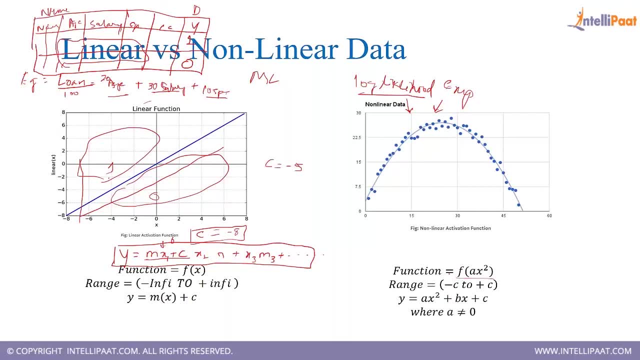 understanding using some other functions available where our neural nets understand that because of the activation function. the main intention of introducing you with linear and non-linearity data is to understand the trends of the data available there first of all, and how neural networks tackles this linear and non-linear data. okay, it learns, based on the quadratic functions. 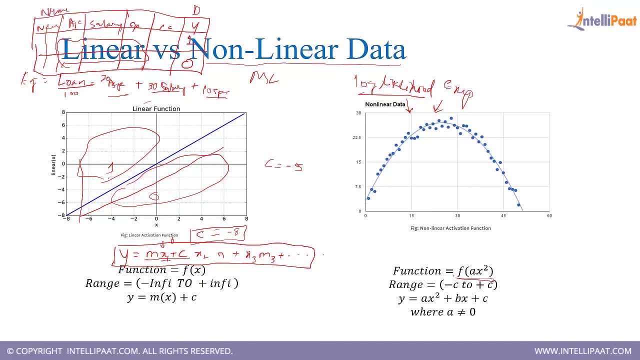 here. so here it is like simple: you have a squared here so that the the graph would look like different. you don't have a slow factor. if you have that, it is like a slope of a parable or something. you have a particular function for it. similarly, neural nets understand each data either. it can be. 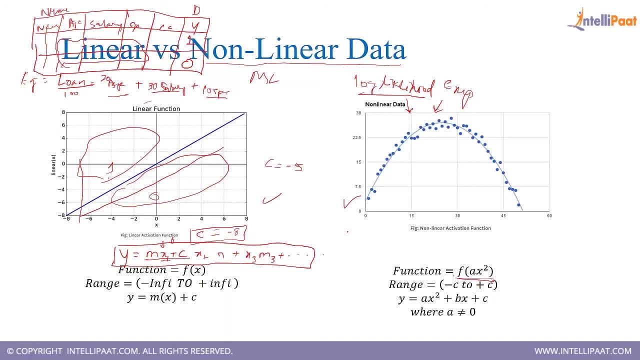 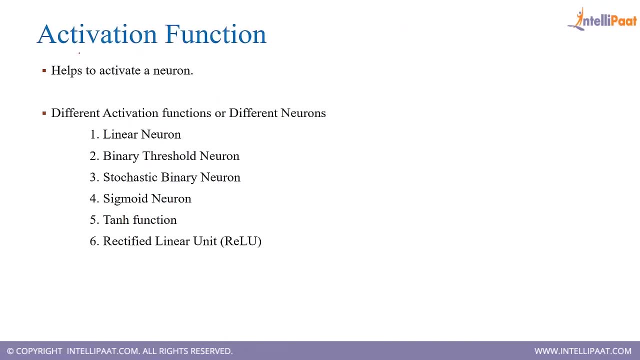 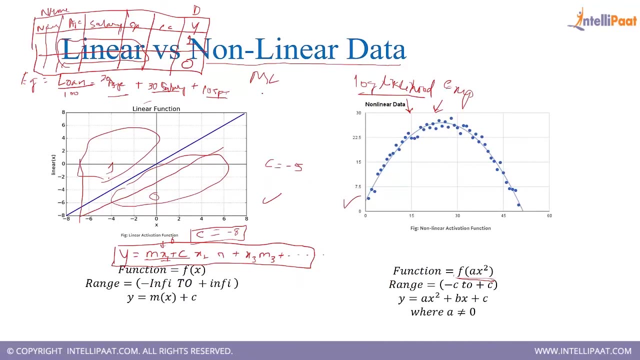 a linear or non-linear, using activation functions. activation functions are the one which we will be looking here based on. because of this, you you will be able to tackle both linear and non-linear data. okay, that is where, most important thing, people will ask in an interview that saying neural net. 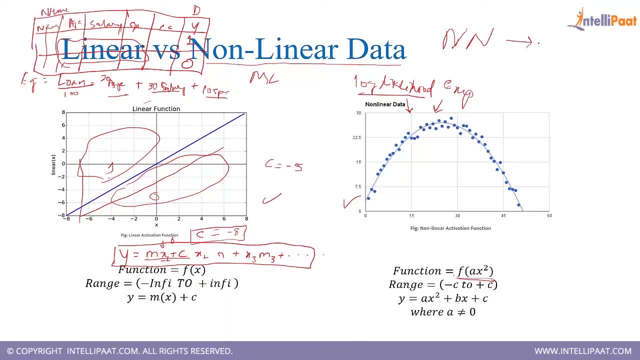 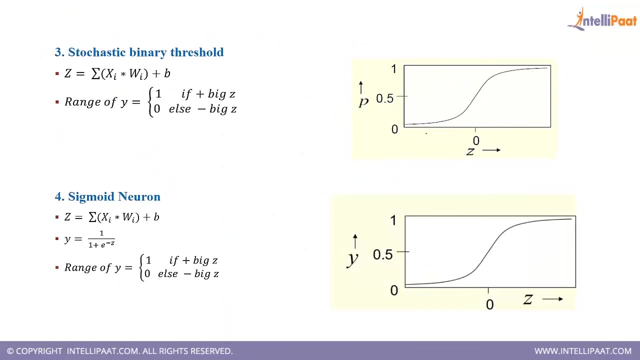 neural net how it handles, uh, linear and non-linear data. you can say that using activation function. how it does that, we will look in when we go here. this is your non-linear data. this is your linear data, got it? this is your non-linearity. it tackles both when it when it comes to the activation. 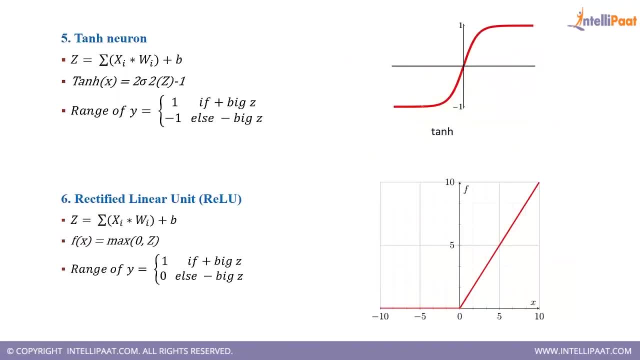 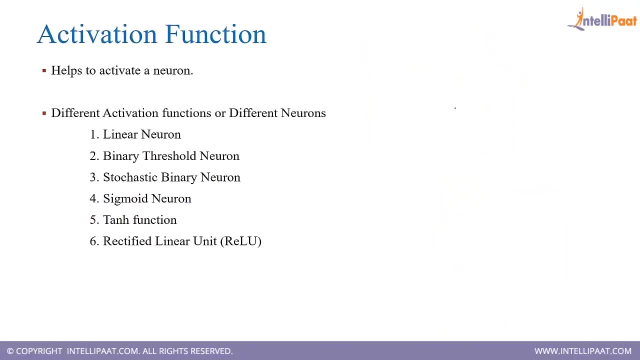 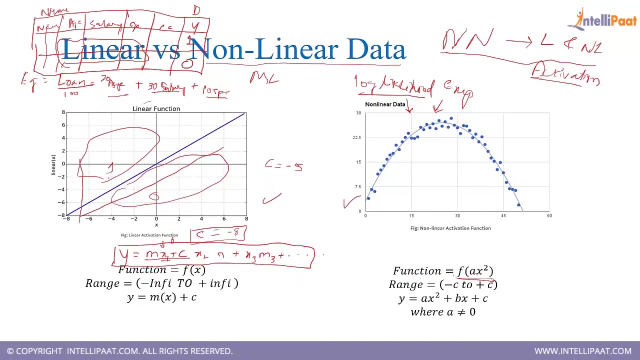 function because of this reason. this is your non-linearity. this region, i mean this reason for that- it handles both activation, linear and non-linear data. okay, just remember the one thing: linear, uh, neural nets handles both linear and non-linear data using act because of the activation part, that's all. 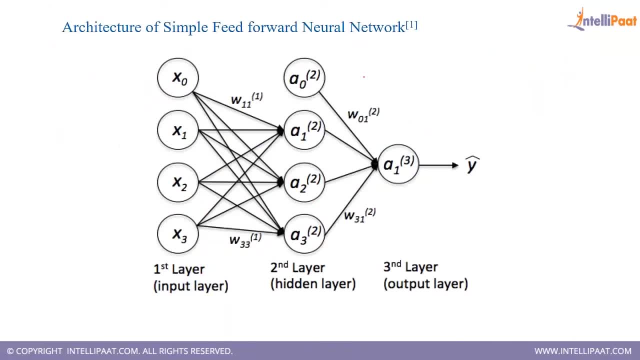 going further ahead. one of the important aspect is understanding the architecture of a feed forward network or simple neural network. what actually is, uh, your feed for? uh simple neural network consists of? It's the input value, the input value and the output value. This is all your inside your box, which takes as your simple neural network. 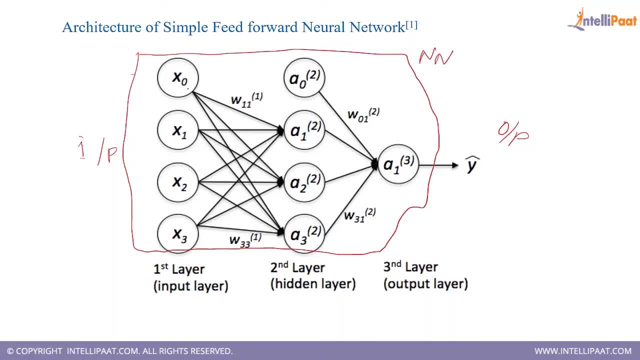 What happens is, as we saw earlier, each input value is associated with its weight in order to pass on to the next level. This is your next layer, right? this is the input layer. this is your middle layer, or hidden layer, when we are the summation of all input tickets: weight: one weight. 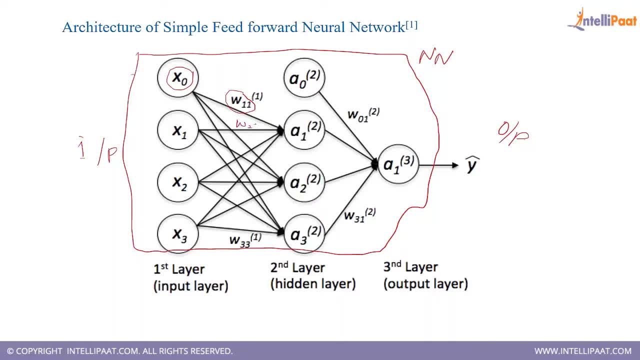 two, two of two, will come here. right, two of two will come here, and then these also go: this one weight, 3 of 3 of 1 actually. so what happens is 3 of 1, 2 of 1 and yeah, so weight are associated with each values will come here. okay, so at this. 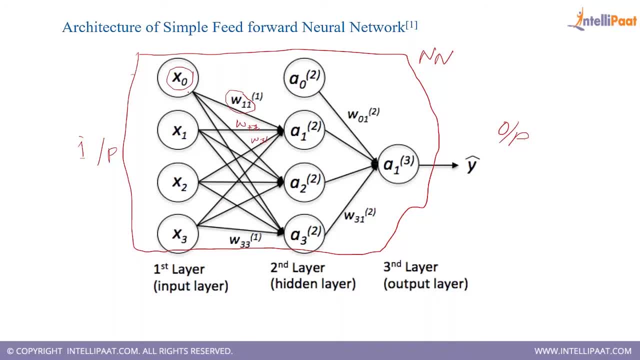 point. what we are doing is we are passing each input to a perceptron. this is a perceptron and the weights associated with that, and each perceptron will have some activation function. okay, each perceptron will have an activation function. at this point you do summation of all weights and their input value. 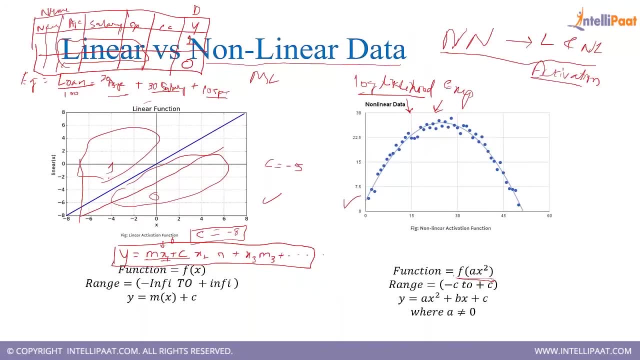 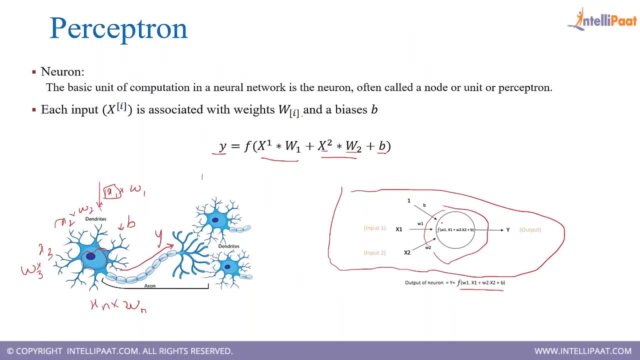 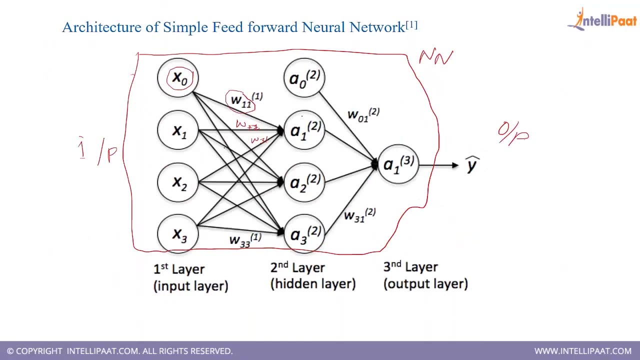 which is this formula, if you remember that which is this formula? weights and input value, with the bias, is your single perceptron. this is a single perceptron. similarly, your single perceptron consist of summation of all those, whichever are coming, whichever are the input involved. right at this point, it comes here and then, at this point, you do activation. 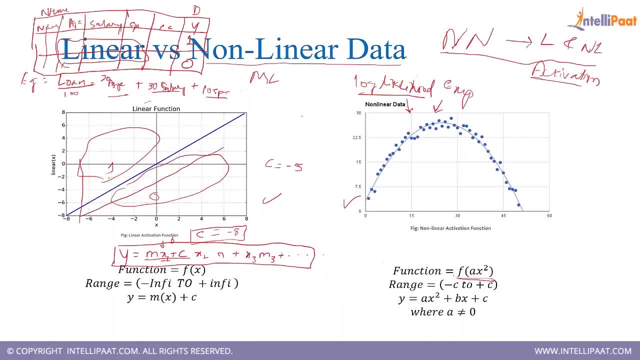 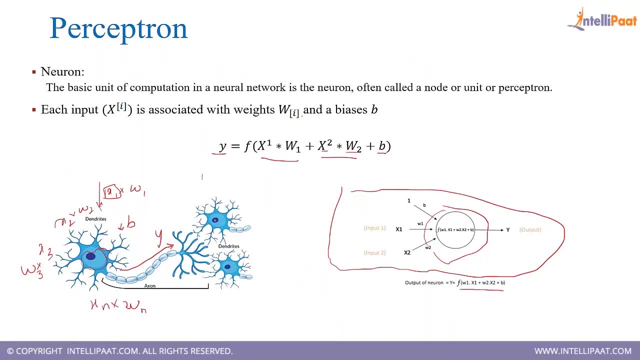 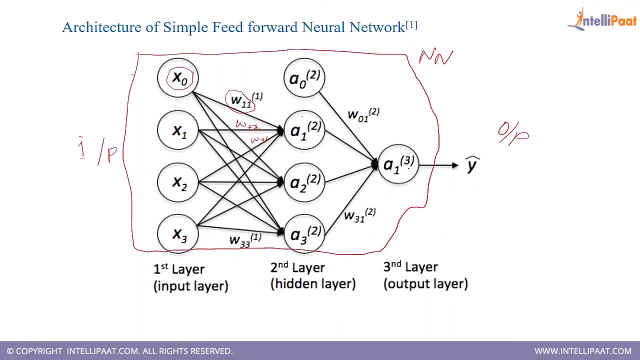 use activation function based on that. remember this one we do. activation function based on that output goes y values, goes to the next layer. so, similarly, this value goes to the next layer, which has another activation function, and then provides you the output. this is the architecture, so I just put on the equation for this one, this perceptron. 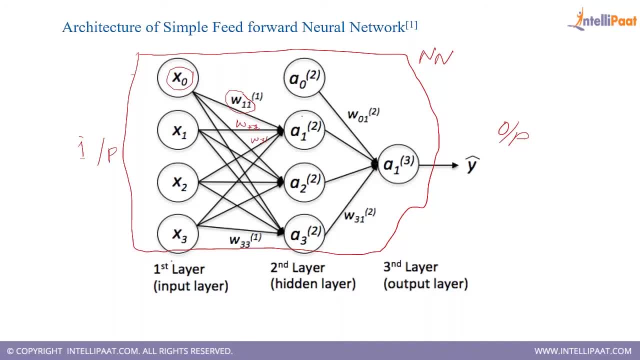 called a1 right. a1 of 2 is equals to function of whatever X naught into weight: 1 plus X- 1 weight, because it is starting with 0 and going to the first one: 0 and 1. 1 and 1 plus X- 2 weight of. 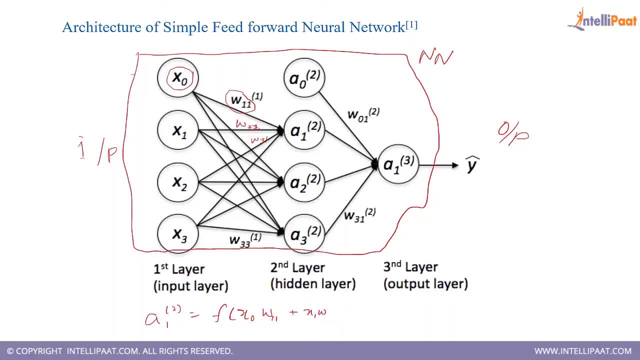 1 and 1 plus X 2 weight of 2 comma, 2 comma 2 plus X 3 weight, 3 plus biases would be the entire function for just this one. see the computation complexity of each layer right, if you see the computation complexity of each layer, you find. 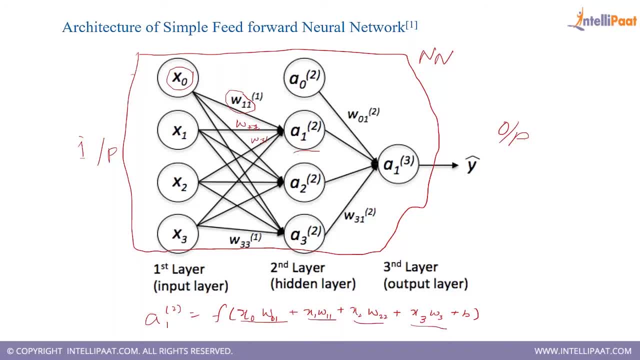 that this computation has to be taken care at each perceptron to get this, and then on top of it you apply either your sigmoid activation function or ReLU or something like that which we will see here. so just that on one perceptron this computation will happen and this information would be passed to the next. 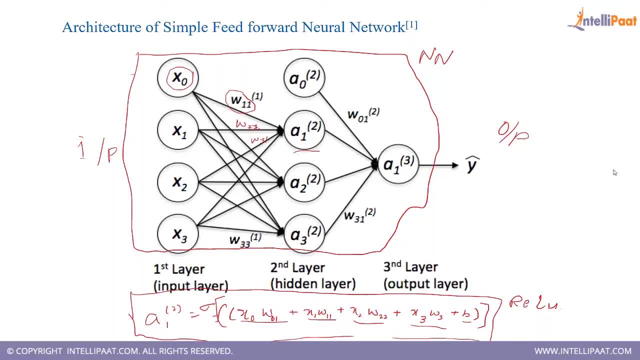 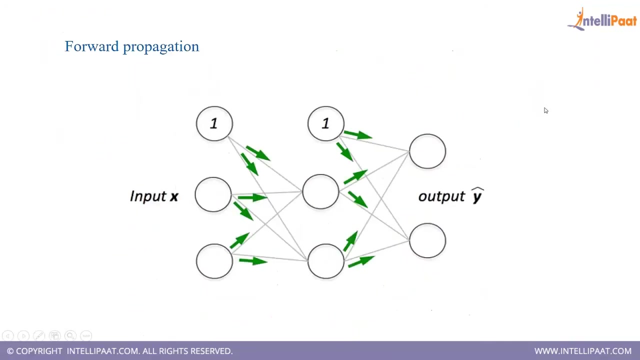 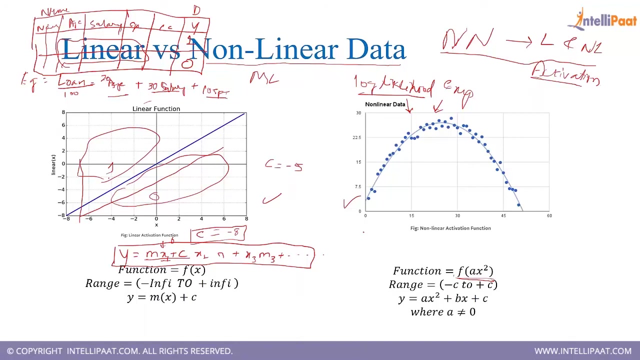 layer for nonlinear data, for example. what we can look for is probably- I'll give you a better example when I go so online, because sometimes what happens is so: sometimes you you cannot have directly get the classification done so and for nonlinear, sometimes what happens is: sometimes you cannot get the classification done so and for nonlinear, sometimes what happens is: 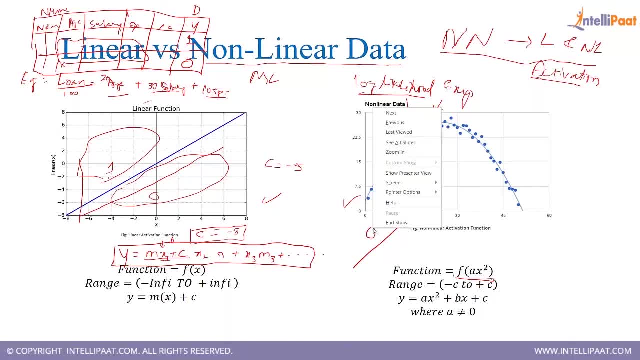 you cannot make a classification between those two different sort of classes. this is one class, this is another class. this is your linear example. nonlinear, what will happen is you cannot directly segregate like this. you need to put in into another dimensional. but this is 2d right, this is two-dimensional sometimes. 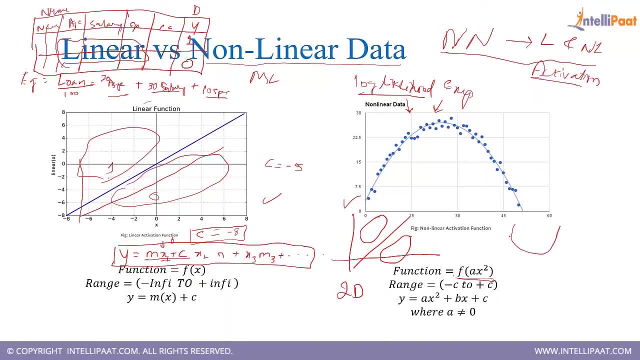 what you need to do. you have data in this format. what you do in order to classify that, you put in another. this is in the three-dimensional. you have something like dimension. I'm bad at drawing. this is your X, Y and Z, probably this. what you are doing is you have a, this parabola at. 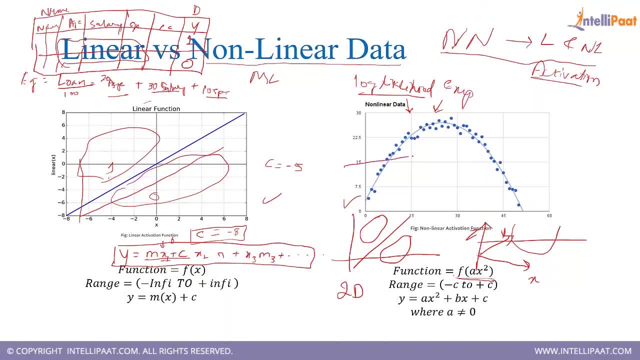 that point. what you can do is: you can do the classification by just putting another line whichever is better than the other line. you can do the classification by just putting another line. whichever is below this area is unto giving a loan. this cannot be given to loan because 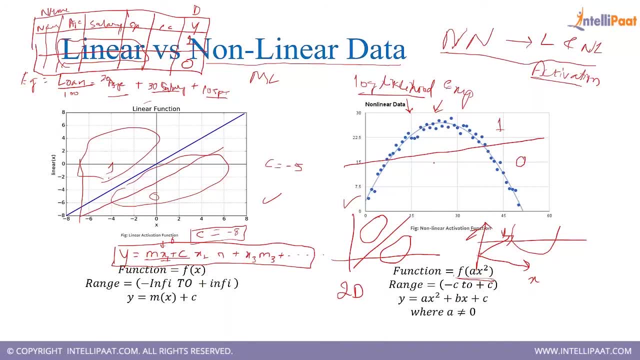 disaggregate that, the line disaggregate that. so sometimes problem would will be like totally different where you have lot of, let's say, miles per gallon and yeah, one example where you can see the direct dependency between two star, which is speed, speed of the car- and display displacement. so you are at a five. 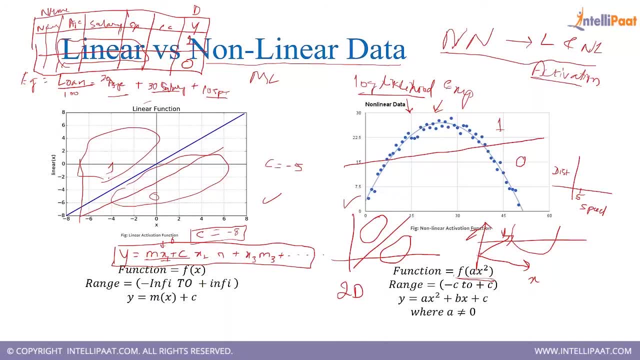 miles per gallon and you suddenly I mean, sorry, five kilometers per mile, sorry about that. and you suddenly put down your brakes. so it would take a displacement of probably like six, my six miles, or not, just six meters, what's a, the unit would be whatever. so at this point it got a displacement. this is your displacement at this point. 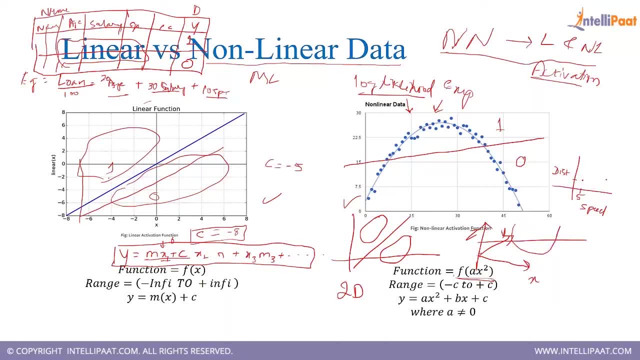 it got your displacement. next is the same thing. next what happens is: you got your. you got your at 10 miles. you stopped by somewhere here earlier, you stopped here and this was the one, okay, so you got something like this linear example as you go further, right, something like this: 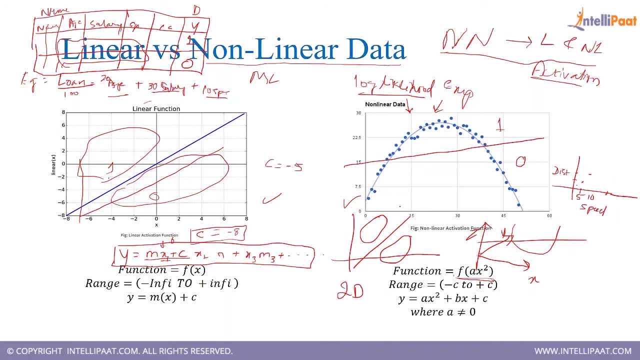 you, this is your, so this is your linear data. actually linear segregation where you trying to predict the value and it gives you a linear problem saying that at 40 miles per gallon, what would be the value so that you predict the y value, that you'll stop by this much, this much. this is your linear example, simple linear. 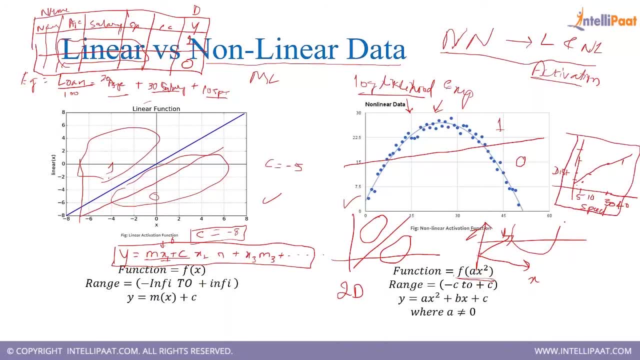 example. but when it comes to a complex problems where you are trying to do where you, you get lot of other parameters and your data would be somewhere, something, something like this. it will not be always a prediction, will not be like this: data will will be somewhere. it starts something like this and then linear. 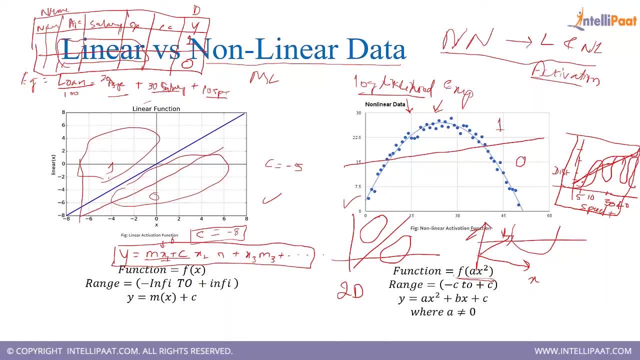 is not it which is called as nonlinear data. when you plot across increasing X, value, Y, how trends would, goes office nonlinearly move here and there. that is what your nonlinear data in in in understanding. I would quote a better example: taking birth help for online, and then I'll let you know. that's where you 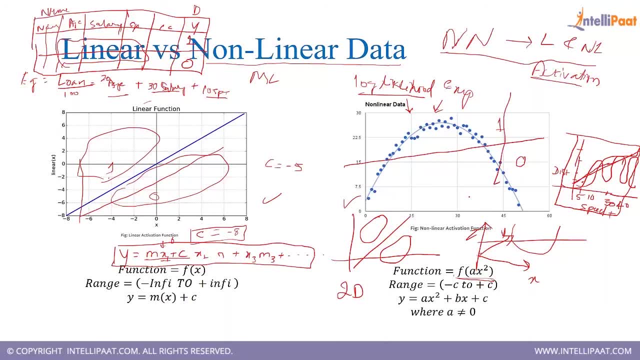 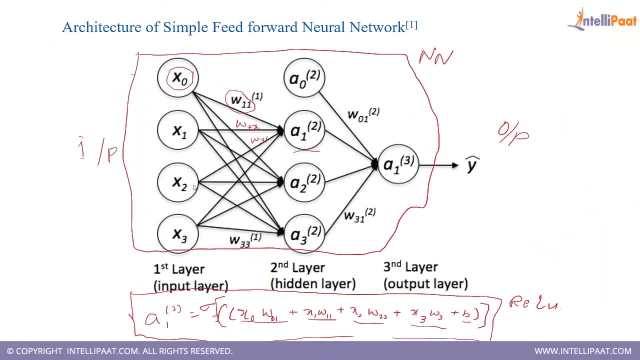 cannot do a segregation for that, so you put in onto another time instead. so, so that it makes you better on the sine curve. okay, yeah, that pretty much thing. this is what it gives. the weightage of these values and then to that of biases would be there, and then activation function. 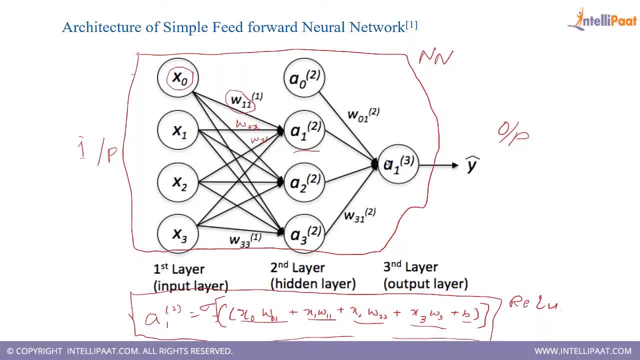 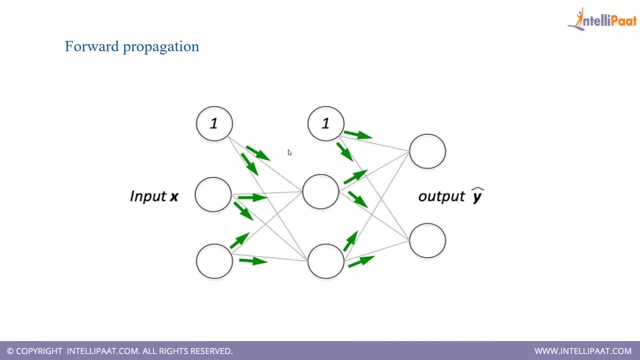 would be imposed on it. then it goes to a next level. okay, that's how you get the y value. so we will look in here. so, forward propagation, what happens is the one value. let's say here, input one is active, it moves on, it moves on. here, you, you get another activation and based on that it will. 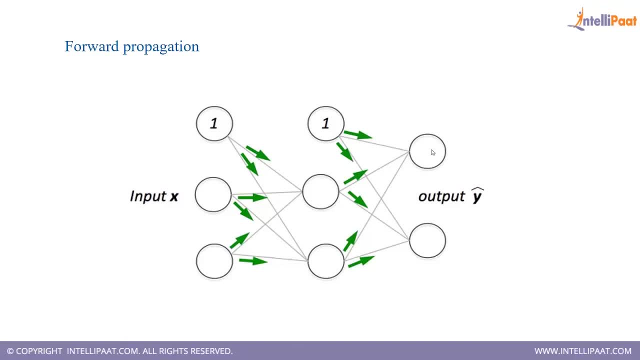 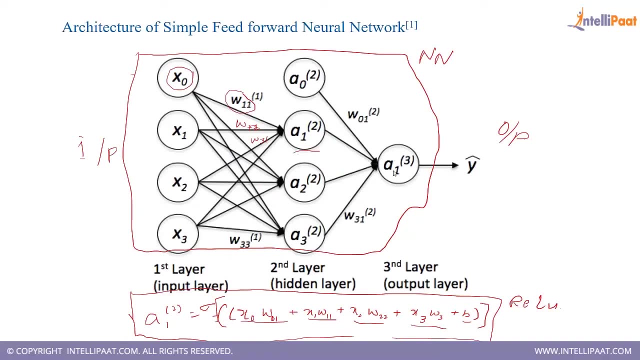 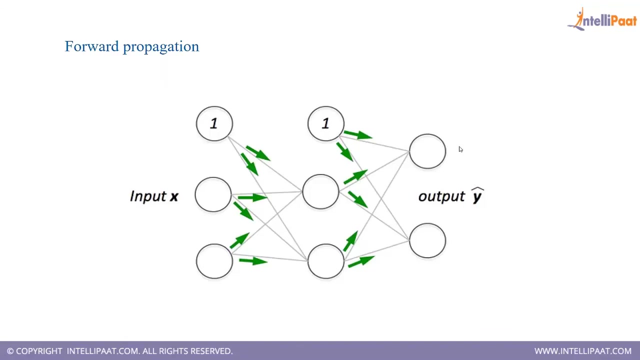 say that either it was one, two or whatever. it was like multi-class classification. the outcome here in, in this scenario, is one. based on that, you say either zero or one, whatever. here also you have two outcomes like that, which can be saying that this is one class distance, one class sort of something. so this is how you can. 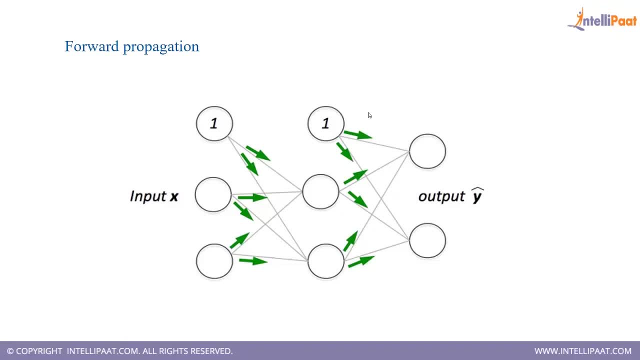 understand that, given input here, one layer of, uh, even activation functions, neurons and all those things which learns the pattern cumulative, all this, this is a cumulative of all. right, it can be this, this will also be linked because, just to make simple thing, it is, it is not. uh, linked it. and then 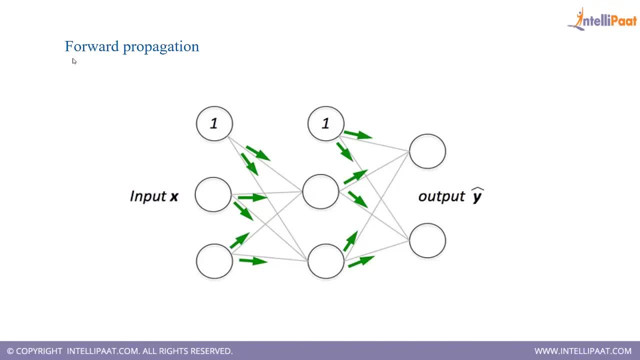 it grows from. from there. this is called as a forward propagation, given that one, it comes here, weights are being updated here, and then it goes to the next level and the values have been available. so next, what is there is? uh, at this point, at these values, what is the activation function we use? either you use sigmoid or either. 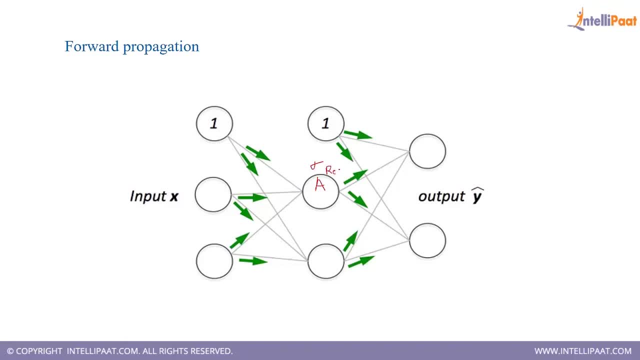 you use uh, tanh, or zelu, which is very famous now, or tanh. what are the various other stuff we will look in here. based on that, it will activate your function. right, accumulating all these things, you get some value and some threshold will be there. above that, it will be one or zero, whatever it pass on to the next. 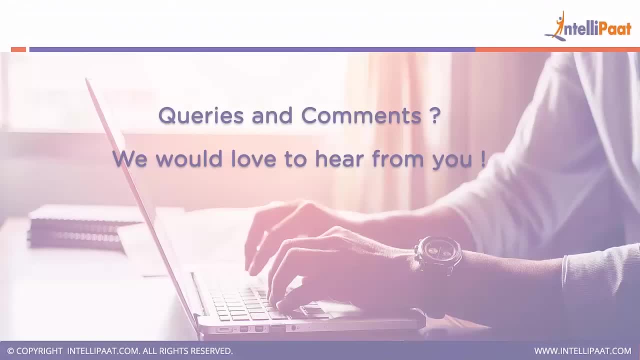 i'm sure you enjoyed learning from this video. please like the video and if you have any doubts regarding this video, please comment us in the comment section. and don't forget to subscribe to our channel for more such informative videos. do look out for other related videos in our